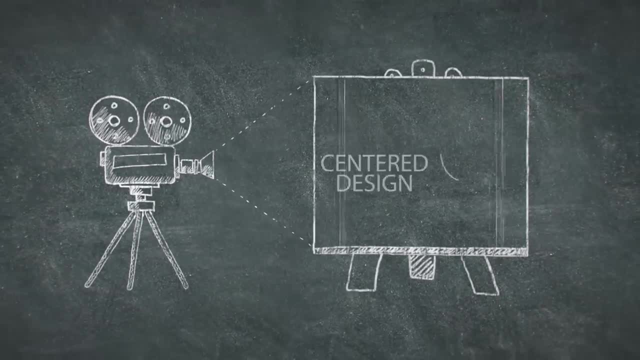 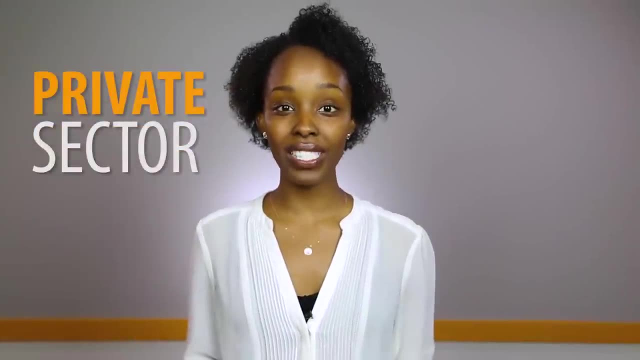 customer or client- Just another buzzword. Let's break down exactly what human-centered design is and why it matters for the global development community. Human-centered design has its origins in the private sector, in fields like user interface design and human-computer interaction. 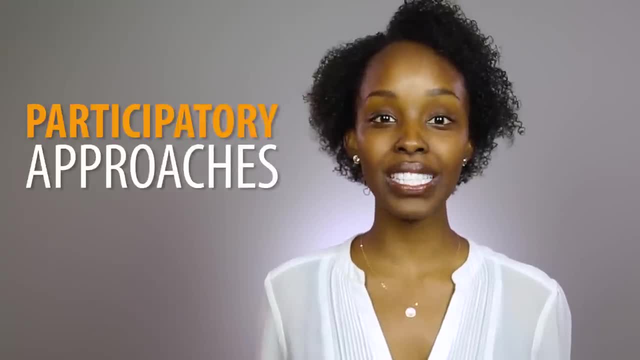 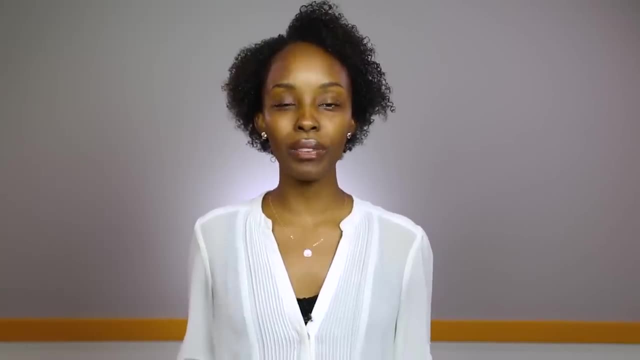 While the development community has long recognized the need for more participatory approaches, the sector still receives criticism for designing for problems instead of designing for people. But what does it mean to design for people? Before creating a solution, development professionals must thoroughly understand the problem. 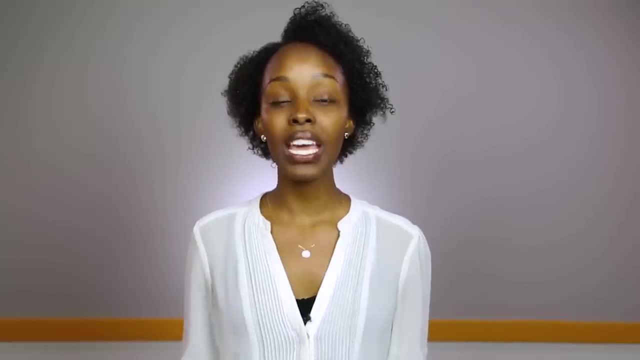 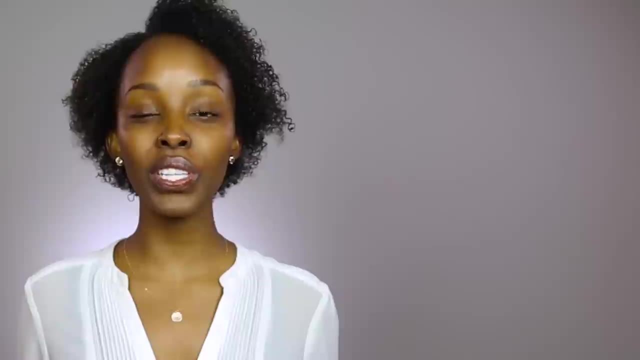 by engaging with communities and individuals, spending time with them, listening to their concerns and understanding the specifics of their lives. This process involves the rigorous collection of qualitative data, which is turned into deep insights about a target audience and the needs of the community. 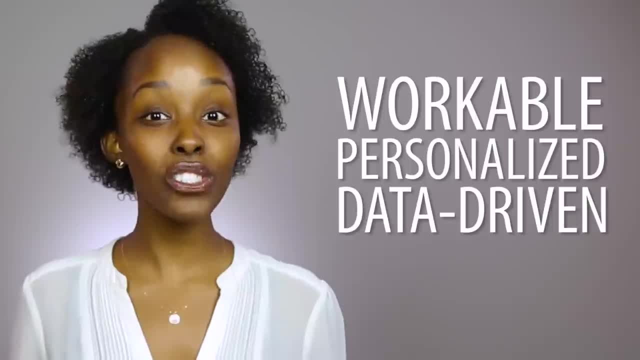 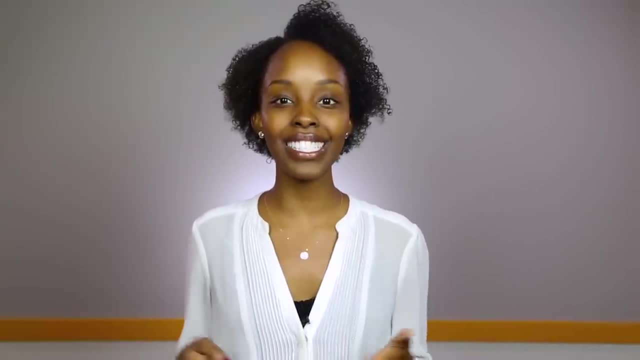 And then it's used to design a set of workable, personalized data-driven solutions for each specific community or country. This means it's inherently built from what works in a given context, instead of trying to adapt an existing solution to fit unique circumstances. 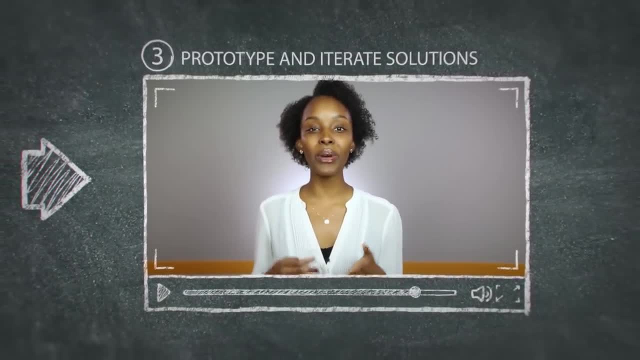 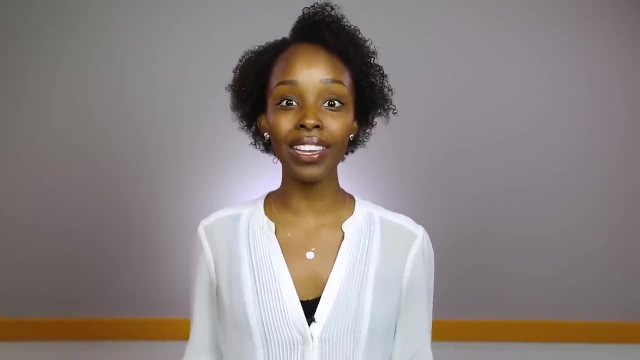 The next stage of human-centered design is prototyping. Prototyping is about getting ideas into the community. to get active participation, Organizations can create a rough prototype that is introduced into the community for feedback and further refined into a pilot. This may seem like a lot of work before you begin to implement a solution. 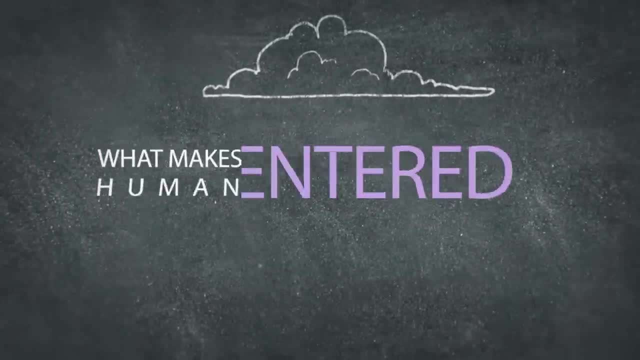 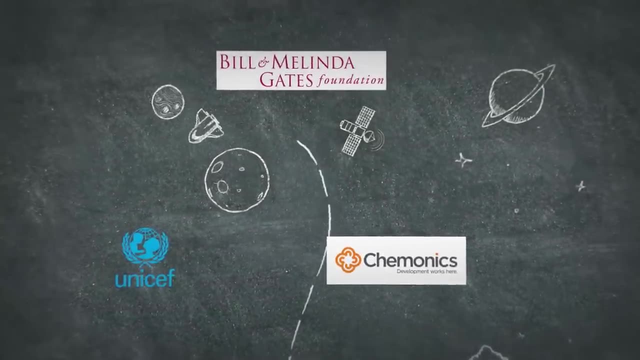 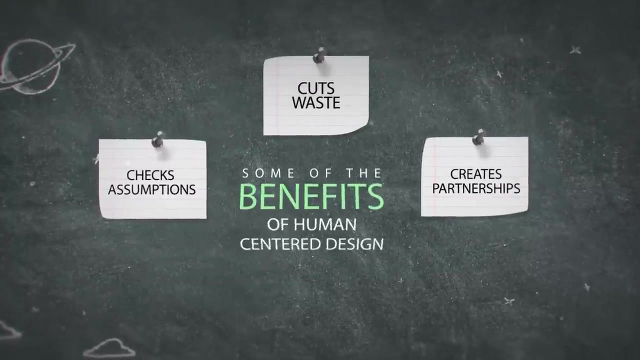 What makes it worth it. Development practitioners are already harnessing this approach at international organizations like UNICEF, philanthropic ventures like the Gates Foundation and private sector development companies like Chemonics. Here are some benefits that they have shared: 1.. 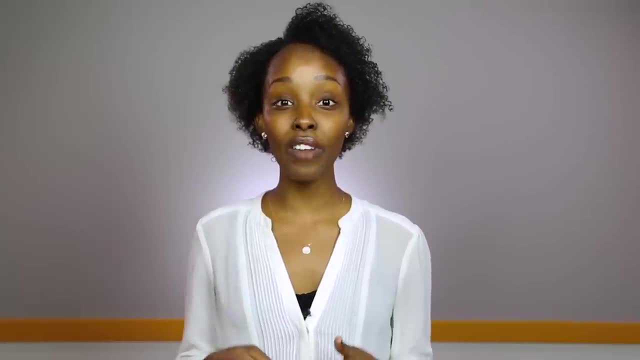 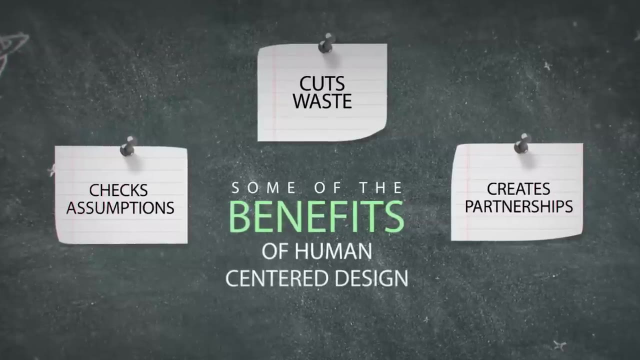 It checks assumptions. Human-centered design helps organizations develop and build on new and ambitious ideas, rather than dismissing them out of hand before they have a chance to prove their worth. 2. It helps us cut waste. Human-centered design is a process that, if executed well, can drastically change the 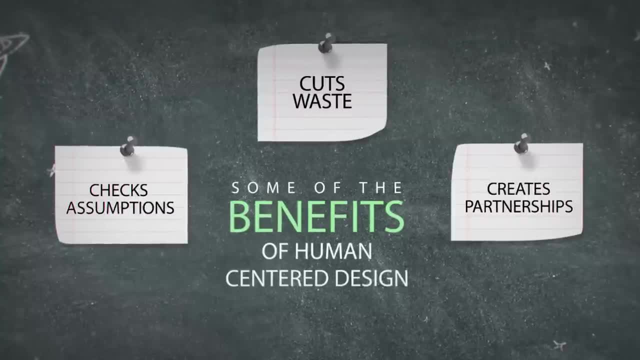 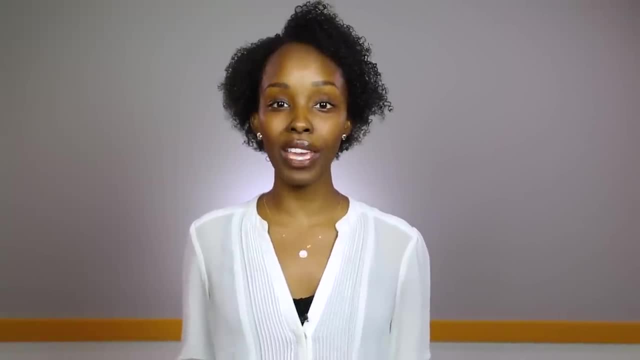 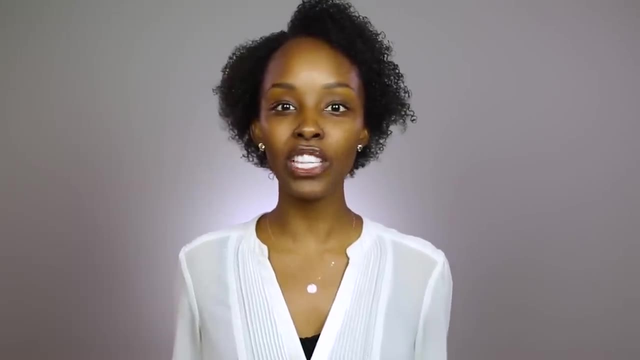 way we use and spend resources. 3. It helps us forge new partnerships. Human-centered design brings together different types of thinkers and makers, people who bring different disciplinary perspectives, cultural understandings and creative abilities. Above all, it pushes us to get into a project with questions rather than catch-all solutions.